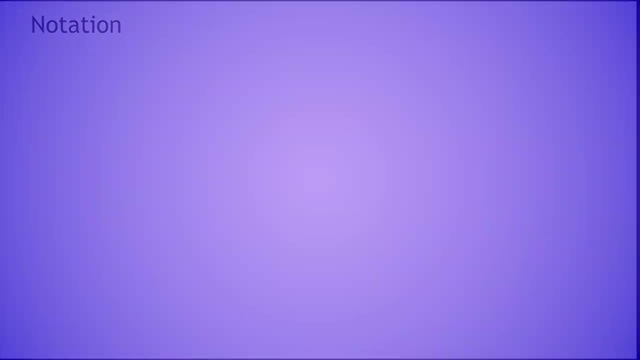 and form an orthonormal basis for this vector space. Let's now explore the fundamental difference between a bit and a qubit. It is always possible to examine a bit to determine if it is in state 0 or 1.. For example, 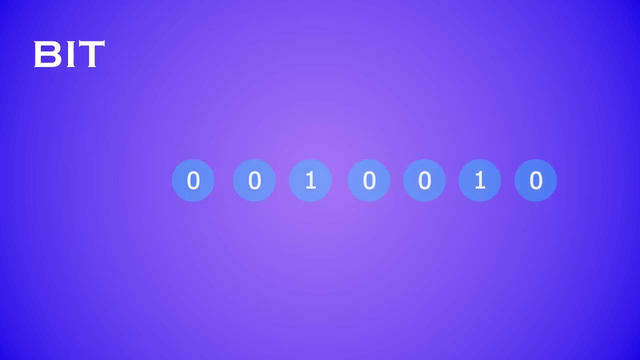 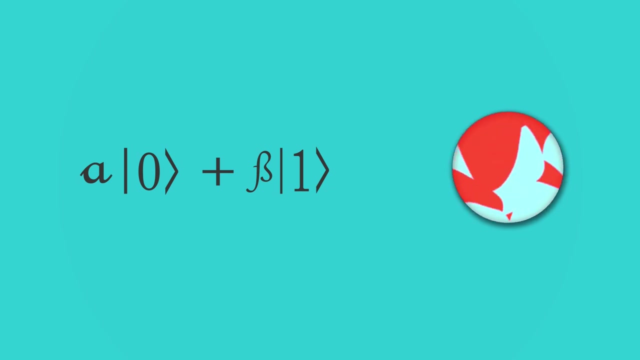 computers do this all the time when they retrieve the contents of their memory. Rather remarkably, it is not possible to examine a qubit to determine its quantum state. For learning the quantum state of a qubit, we need to learn the values of alpha and beta. 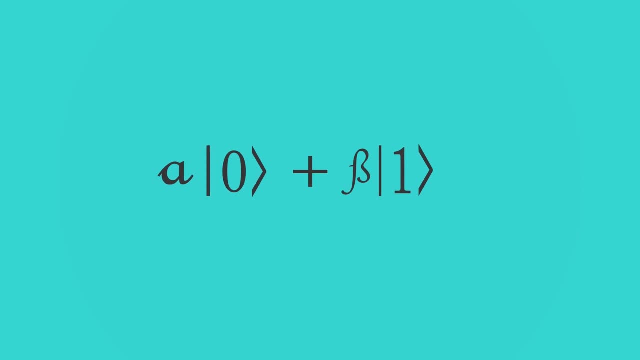 However, quantum mechanics tell us that we can only acquire much more restricted information about the quantum state. When we measure a qubit, we get either the result ket 0, with probability alpha squared, or the result ket 1 with probability beta squared. 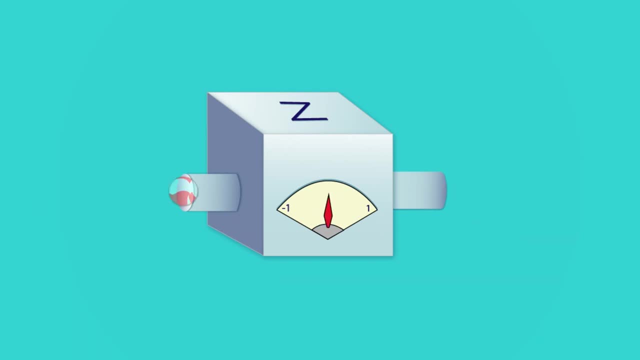 So from a single measurement we will not be able to learn the values of both alpha and beta. Thus, in general, a qubit state is a unit vector in a two-dimensional complex vector space and measurement collapses it into one of the bases. 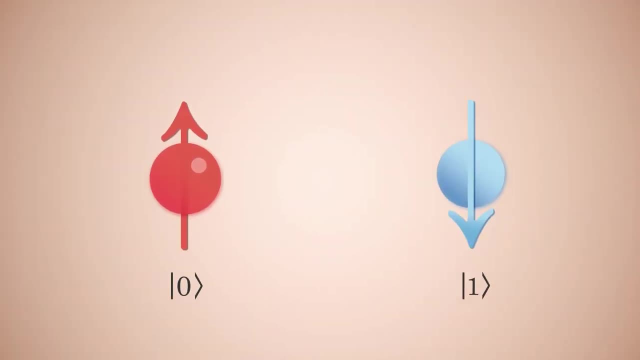 Qubits' ability to be in superposition states runs counter to our common sense. A classical bit is like a coin: either heads or tails. By contrast, a qubit can exist in a continuum of states between ket 0 and ket 1 until it is observed. 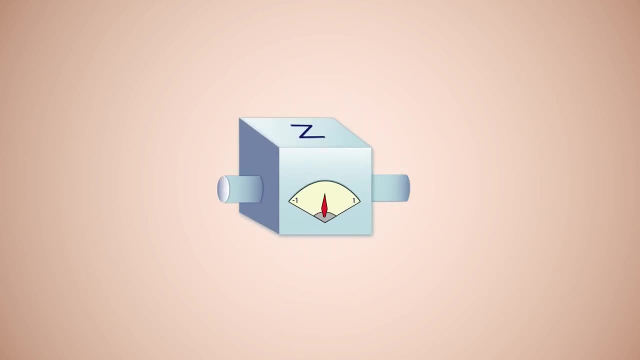 Let us emphasize again that when a qubit is measured, it only ever gives 0 or 1 as the measurement result. probabilistically, For example, a qubit can be in the state which, when measured, gives the result 0, 50% of the time. 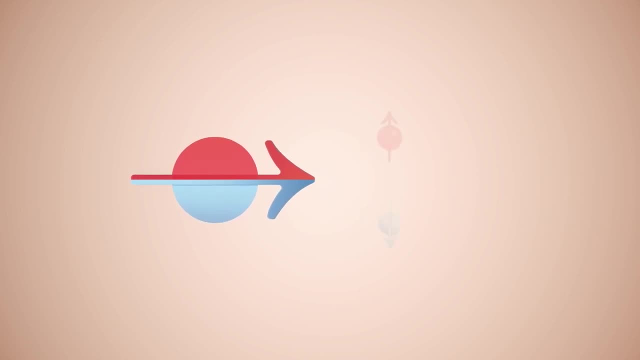 and the result 1- 50% of the time. This state, which is in the same state as the measurement result, can be in the state which, when measured, gives the result 0- 50% of the time and the result 1- 50% of the time. 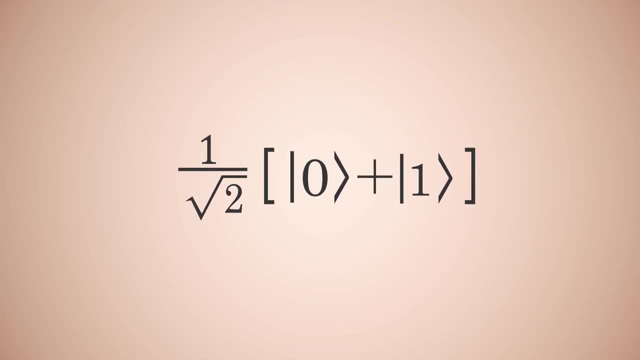 This state, which is in an equal superposition of ket 0 and ket 1, is quite an important quantum state and is sometimes denoted by ket plus. Although qubits seem strange, they are in fact real. Experiments extensively validate their existence and behavior. 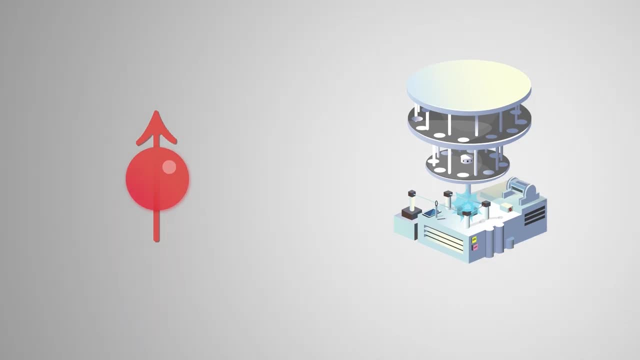 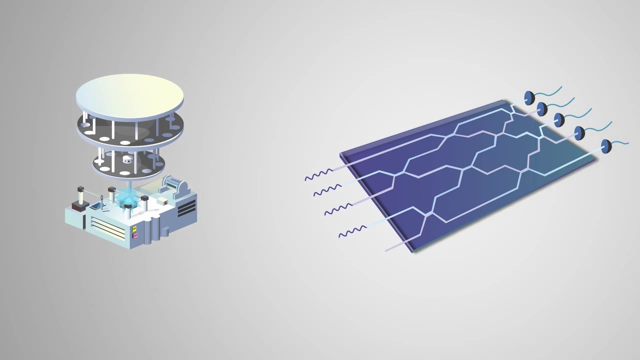 and they can be realized using a wide range of physical systems. In order to get a sense of how a qubit can be realized, let's see some of the ways it can occur: As the two different polarizations of a photon, as the alignment of a nuclear spin in a uniform magnetic field. 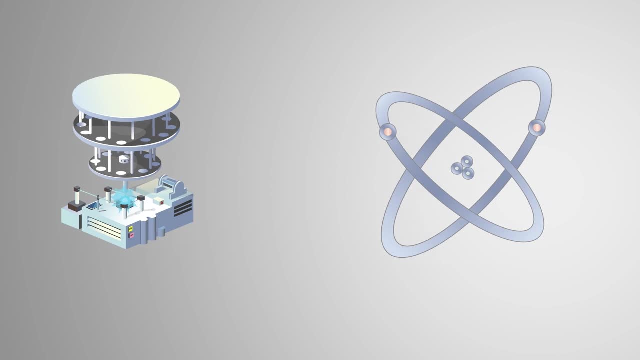 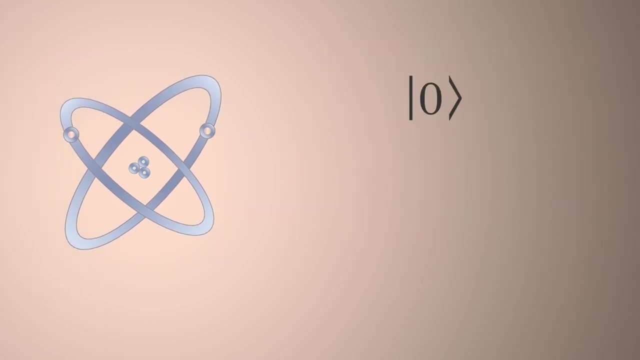 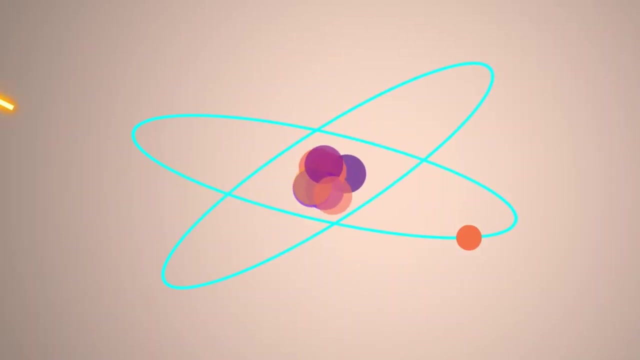 as two states of an electron orbiting a single atom. In the atom model, the electron can exist in either the so-called ground or excited states, which we'll refer to as ket 0 and ket 1 respectively. By shining light on the atom with appropriate energy and for an appropriate length of time. 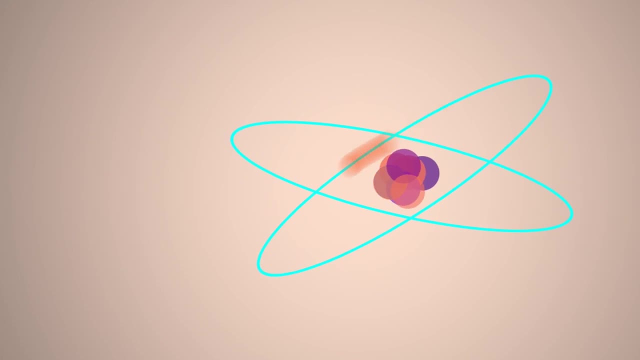 it is possible to move the electron from the ket 0 state to the ket 1 state and vice-versa. But, more interestingly, by reducing the time we shine the light, an electron initially in the state of ket 0 can be moved halfway between ket 0 and ket 1,. 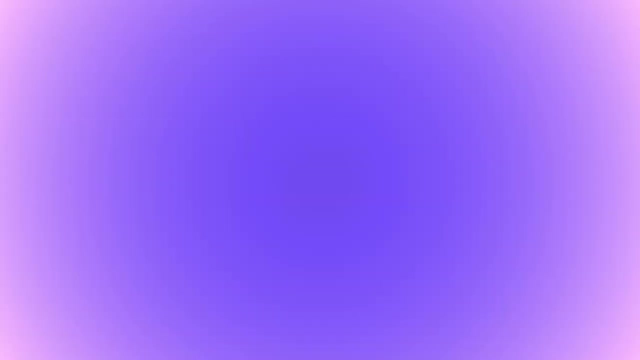 into the ket plus state. Historically, a great deal of attention has been given to the meaning or interpretation that might be attached to superposition states and to the inherently probabilistic nature of observations on quantum systems. However, for almost all practical purposes related to quantum information processing, it is not. 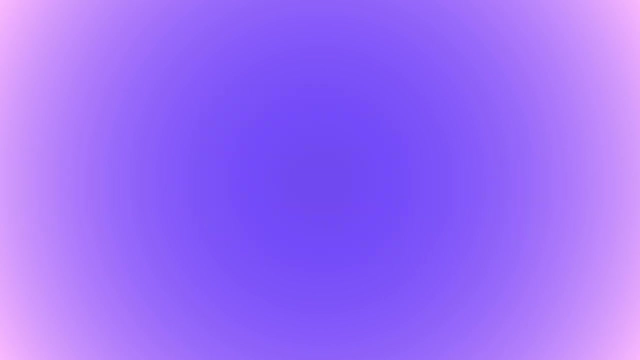 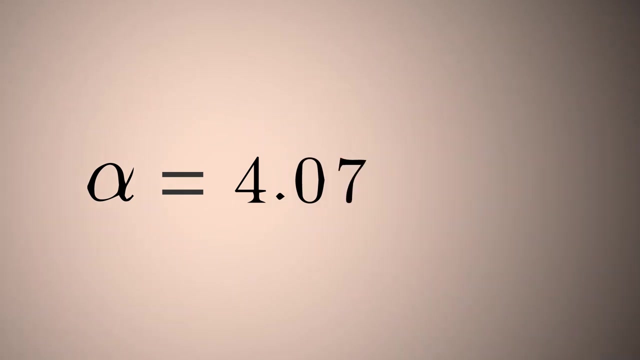 necessary to concern with such discussions. how much information is represented by a qubit? paradoxically, we can do infinite binary expansion of values alpha and beta, so in principle it could store infinite information. however, this conclusion turns out to be misleading because of the behavior of a qubit when observed. recall that measurement of a qubit will give only 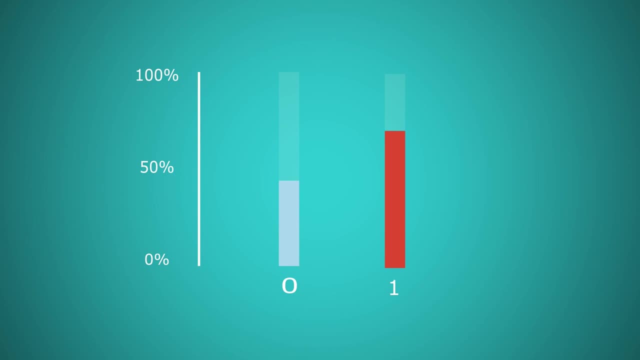 either 0 or 1. furthermore, measurement changes the state of a qubit, collapsing it from its superposition of cat 0 and cat 1 to the specific state consistent with the measurement result. for example, if the measurement of cat plus gives 0, then the state of the qubit after measurement will be cat 0. why does this? 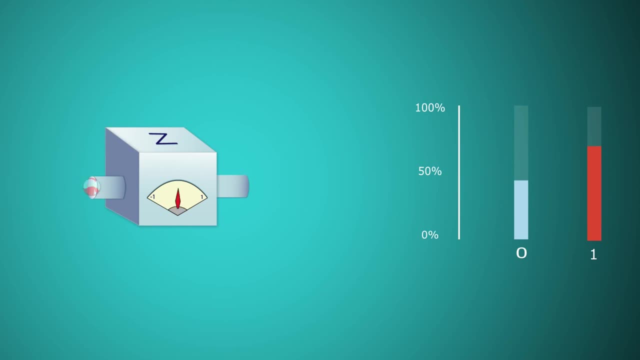 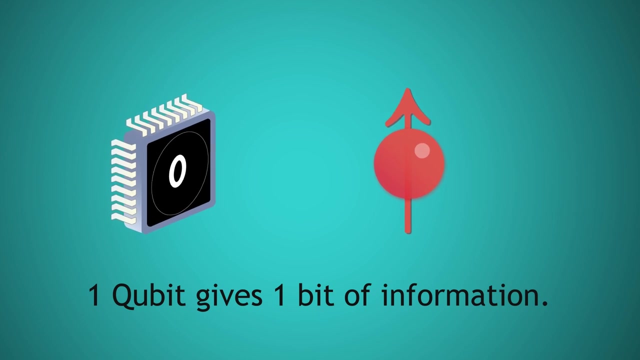 type of collapse occur, nobody knows until now. we simply accept it as a law of nature and included as one of the fundamental postulates of quantum mechanics. what is relevant for our purposes is that from a single measurement, one obtains only a single bit of information about the state of the qubit, thus resolving the apparent.